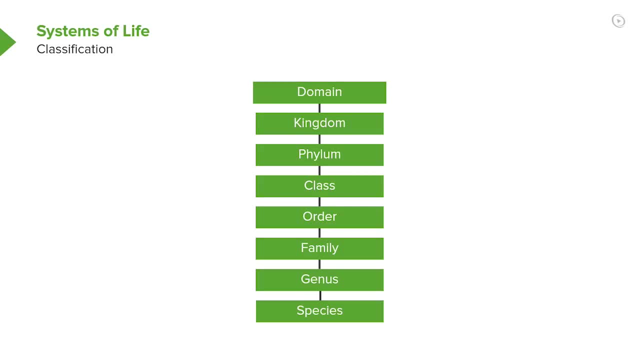 On the screen you can see one hierarchical scheme That is used to describe essentially every living organism on Earth, starting at the top, with the most broad view, and narrowing down as we go down through the names. Domains, of course, relate to the very, very broad regions relating to living systems. 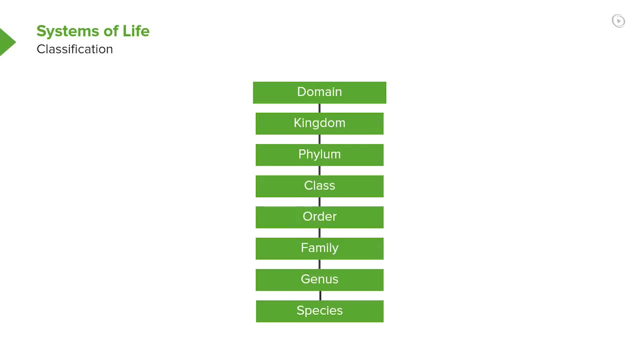 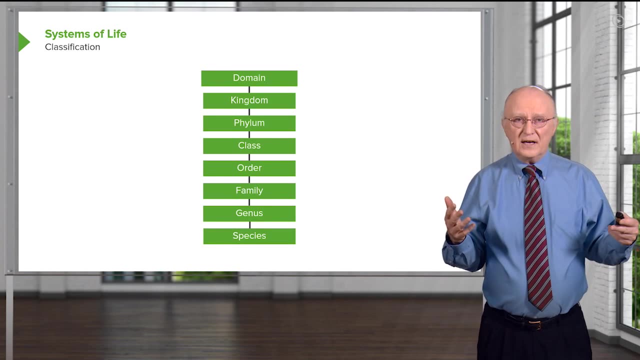 Kingdoms are a subdivision of that, and phyla are a subdivision of the kingdoms, followed by class, order, family, genus and species. Now it's important to recognize that every life form on Earth is different. Every life form on Earth can be described by this hierarchical system. 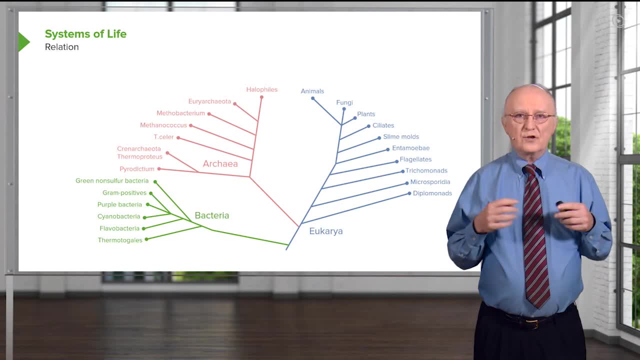 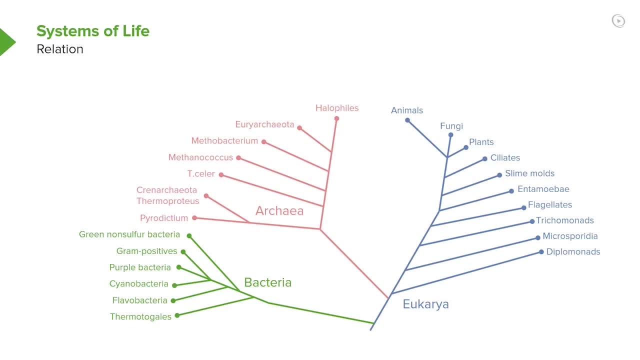 Another system for organizing life is that shown on the screen, based on evolutionary distance. We think that all life on Earth ultimately came from one primordial cell, and that one primordial cell evolved and gave rise to all the life forms that we see today. 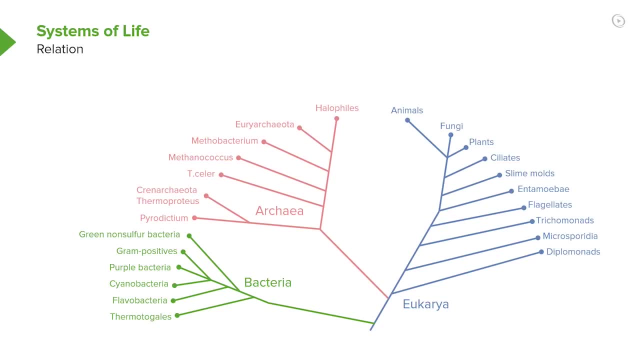 This plot shows as lines the evolutionary distance each living system is from that primordial cell and, by extension, how far each living system is Evolutionarily from each of the other systems. on the screen On the lower left we can see bacteria. 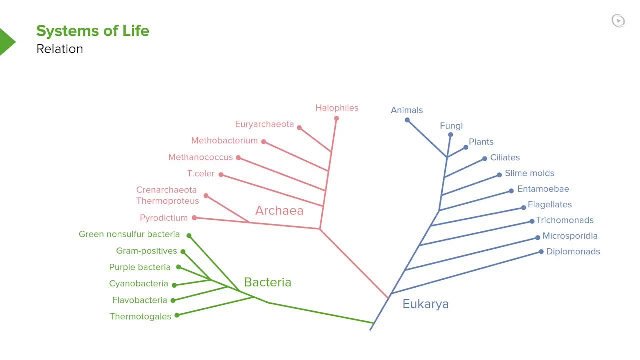 Bacteria, of course, are the single-celled organisms that contain no organelles. They're very simple in their structure and they're very tiny. One of the ways people view bacteria is as a bag of enzymes and nucleic acid. 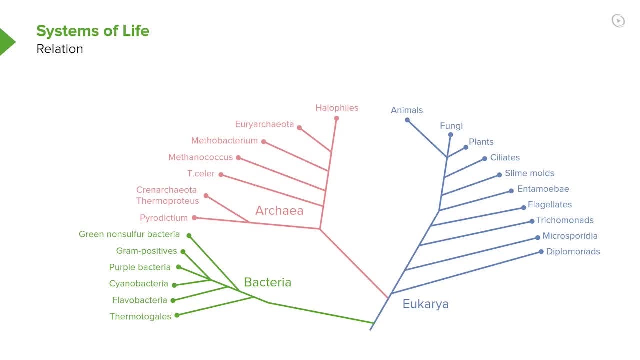 And that's about what we find in bacteria. The Archaeans are the more recently described types of life, and they actually exist in some of the world, One of the most inhospitable places on the planet, Environments that other cells would find toxic, the Archaeans find home. 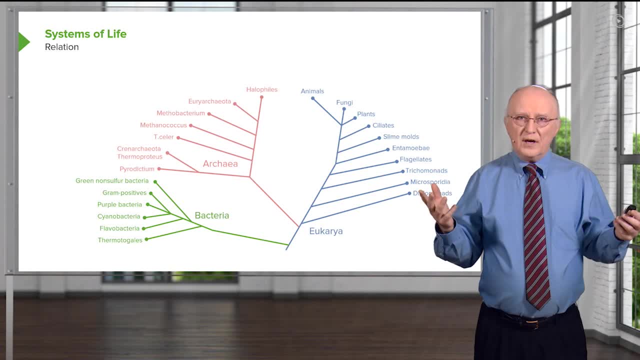 Like bacteria, they're very simple as well. The Eukaryotes shown on the right include the multicellular organisms we see on Earth. This includes the animals, the fungi, the plants and many other multicellular and a few unicellular forms as well. 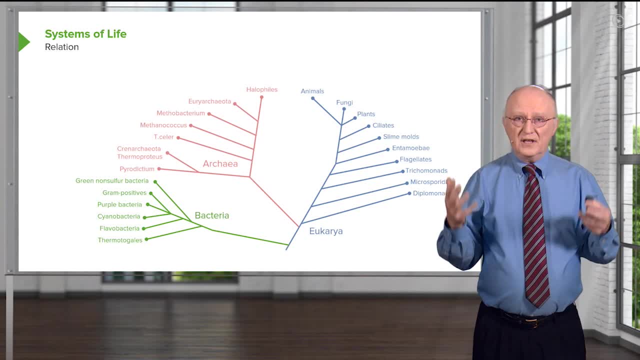 One unicellular form we see in the Eukaryotes includes the yeast makers of bread and ethanol. Now, the Eukaryotic cells differ from the Prokaryotic cells and the Archaean cells in, first of all, generally being considerably larger than them.